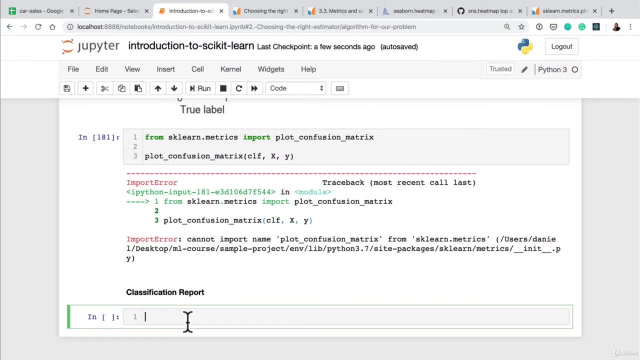 So the final classification model evaluation metric we're going to have a look at is a classification report. And now, really, a classification report is more so a collection of different evaluation metrics rather than a single one. So that's where the report comes from. 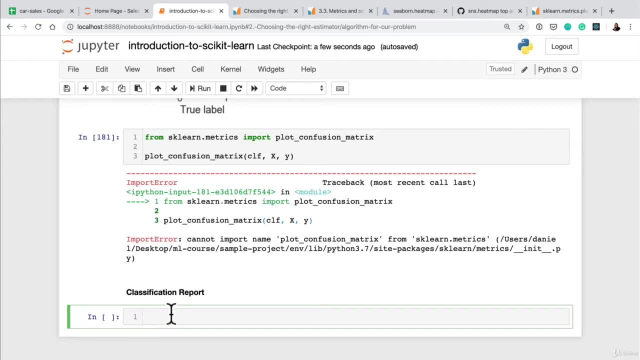 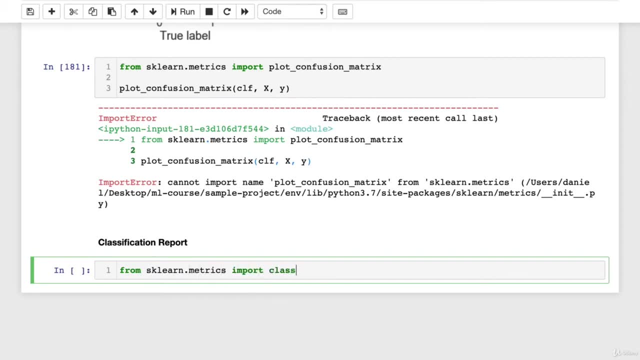 It's going to report back of a number of different parameters evaluating our classification model. Let's see one in action. So, from sklearnmetrics import classification report To do it, we just pass it some true labels, aka ytest, and some predictions. So, once again, 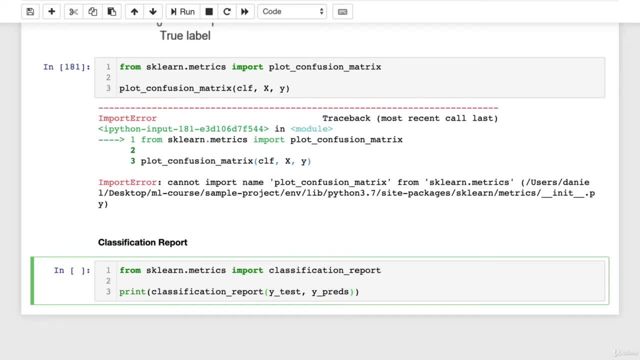 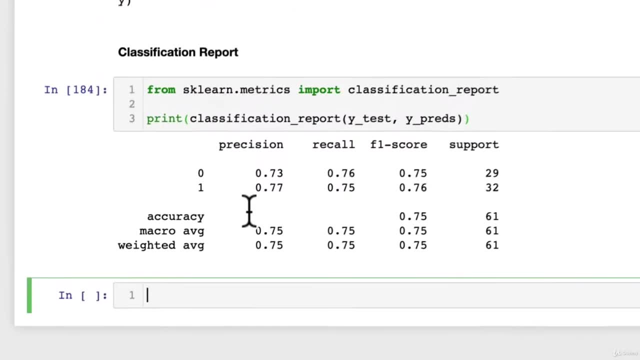 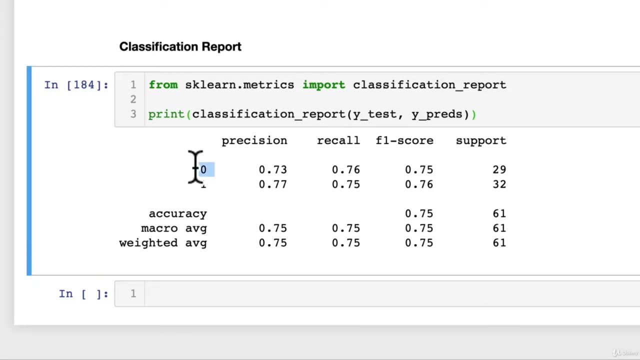 this evaluation metric is just comparing the true labels of our data versus the predictions that our model has made, So let's see what happens here. All right, There's a fair few things going on. We've got precision recall F1 score support zero. maybe that's for the class. 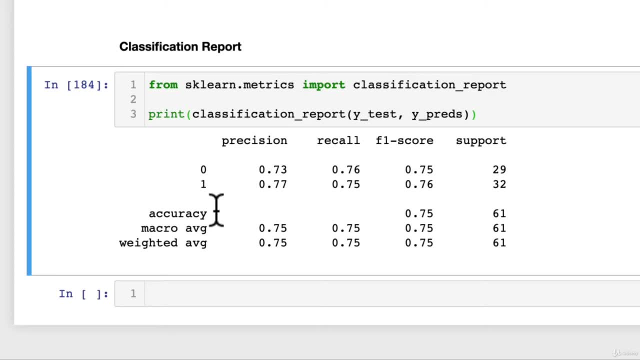 zero for not heart disease. one, Maybe that's for heart disease. If we come down, we've got accuracy 0.75, macro average, weighted average. Hmm, What's going on here? Well, let's go to our keynote and have a look. 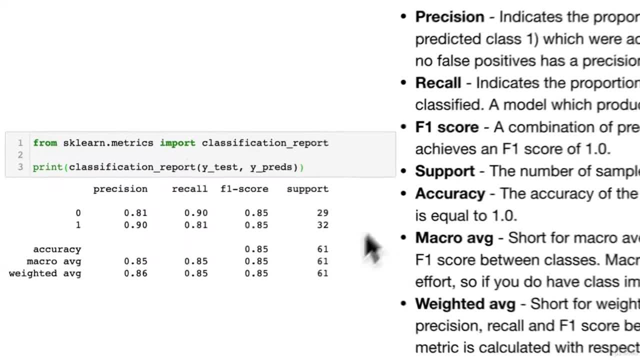 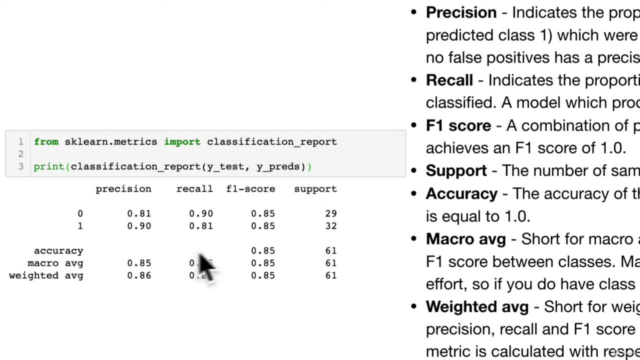 at our classification report, anatomy. So over here we see we've got the same thing. So just import classification report. We've done one on the test labels and the predictions- some slightly different numbers here, what's in our notebook, but that's okay. 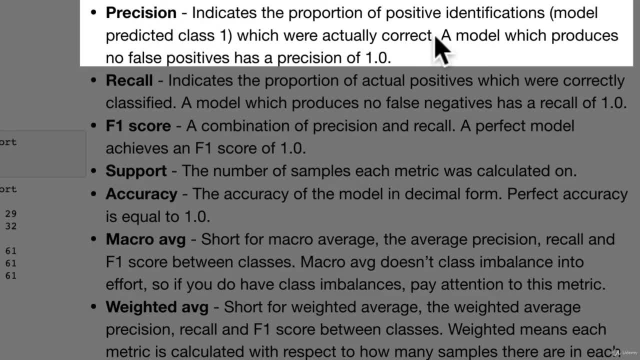 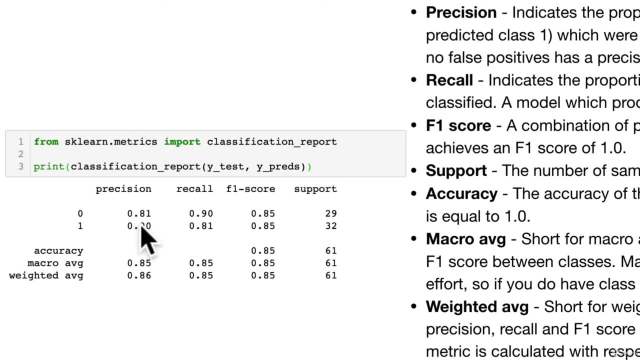 So what's precision? Well, precision indicates the proportion of positive identifications, so, aka the model predicted, class one, which were actually correct. Now, a model which produces no false positives has a precision of one. So that's where we can see our precision scores. If the model produced 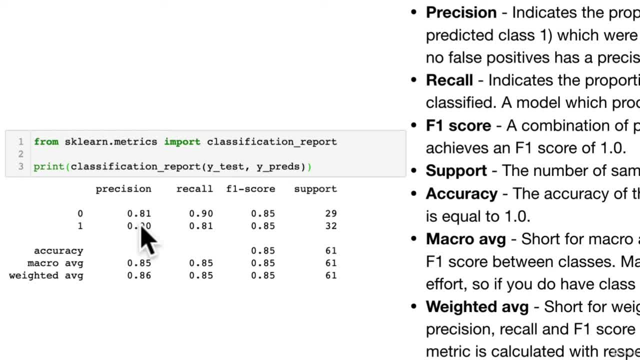 no false positives and we know that our model hasn't because we've looked at the classification or the confusion matrix and we've seen it confused on some examples and it's predicted them as false positives. So our precision scores are a little bit lower than one. 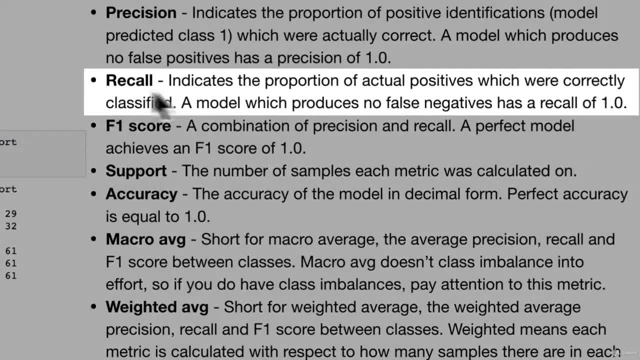 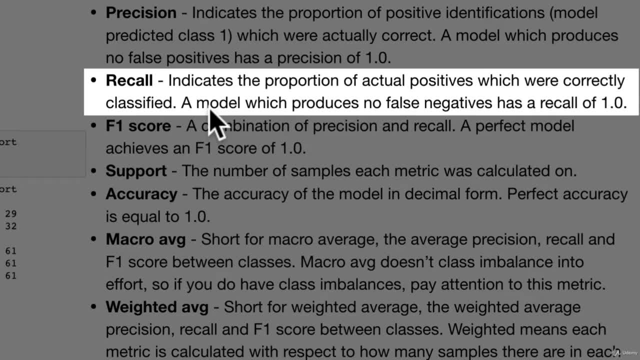 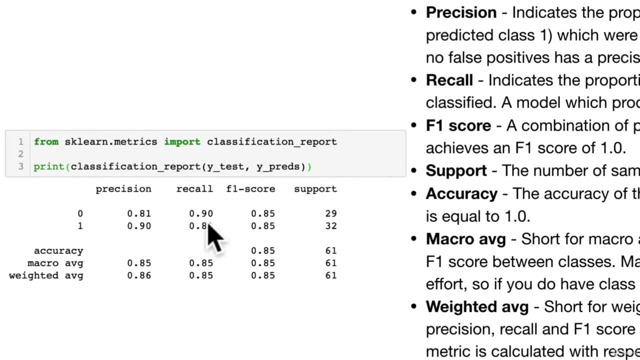 Now the next one is recall. So recall indicates the proportion of actual positives which were correctly classified. Now a model which produces no false negatives has a recall of 1.0. And again we know from our confusion matrix that this isn't the case, So our recall is a little bit lower. 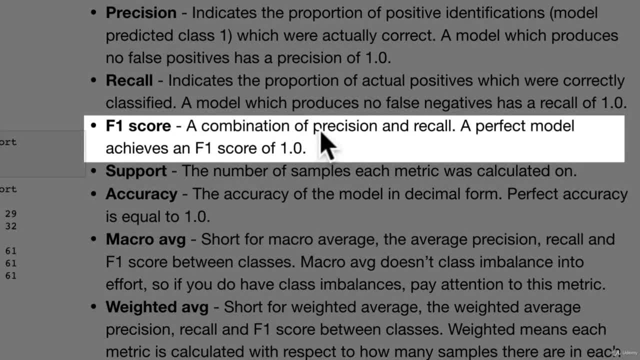 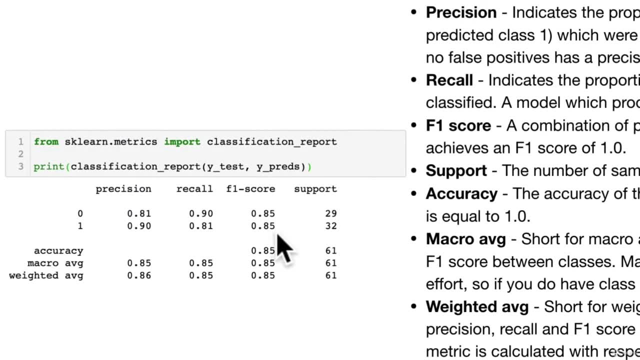 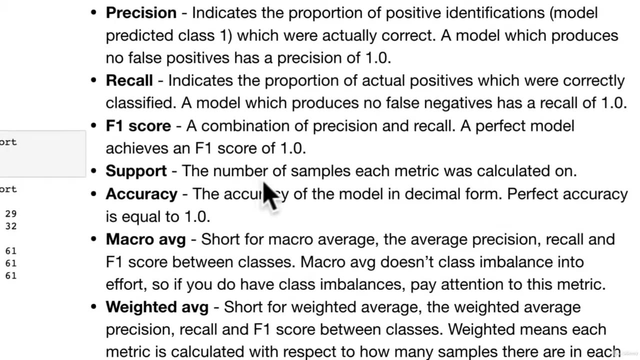 Now our F1 score. a combination of precision and recall- A perfect model- achieves an F1 score of 1.0.. Okay, So we're going to see our F1 score. F1 score is not 1.0, but it's still relatively high. Then, if we go support the number of samples, 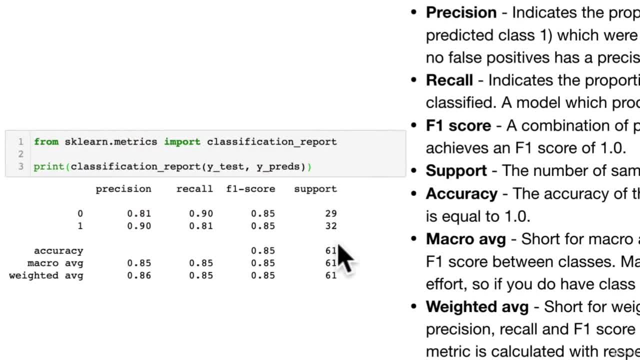 each metric was calculated on. So we see here: so this means we look at this 29.. So we look at that. that's for zero. Now down here it's 61. So that means that these metrics here were calculated on. 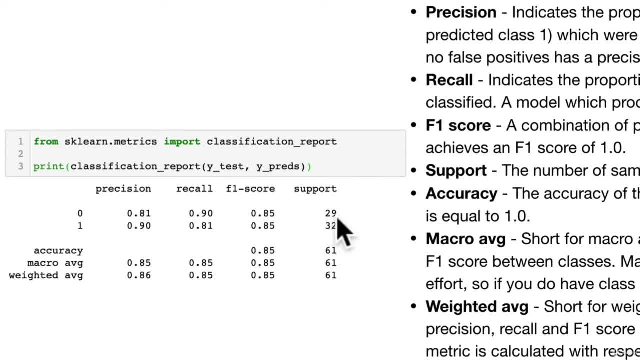 61 different samples, And these metrics along here were calculated on 29 samples which had the class 0. And that this one is 32 with the class label 1, aka has heart disease, And so if you total these up, 29 plus 32, you get 61.. Now accuracy. we've seen that before. This is just the accuracy of 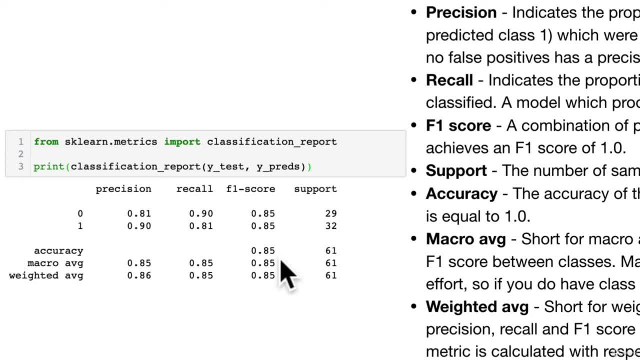 the model in decimal form, Perfect accuracy is 1.0, aka our model is making predictions right 100% of the time if its accuracy is 1.0. Then we have a look at macro average. Now what is that? It's short for? 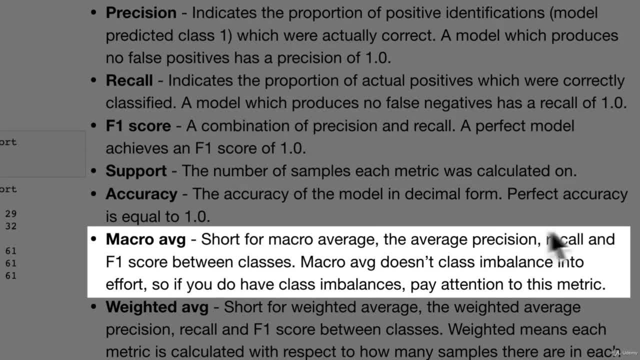 Macro average, as you may have guessed. So it's the average precision, recall and F1 scores between classes. Now the key here is macro average. doesn't take class imbalance into. This should be effect into Or account. So pretend this is account. So if you do have class imbalances, 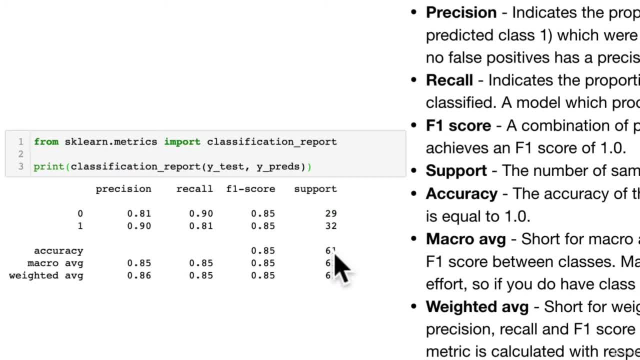 pay attention to this metric. Okay. So in our case, what is a class imbalance? Well, if you look at our example, we don't have class imbalances here. Why is that? Well, because we have relatively the same amount of samples with class 0 and class 1,. 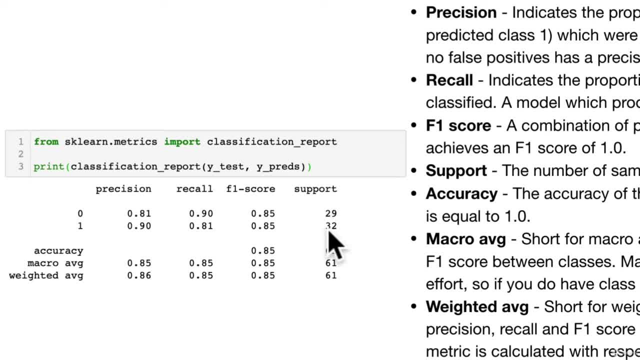 meaning we've got about 50-50 split here. It's not exactly 50-50, but it's not like we have 60 examples of class 1 and 1 example of class 0. So we've got about 30 in each. So if you did have 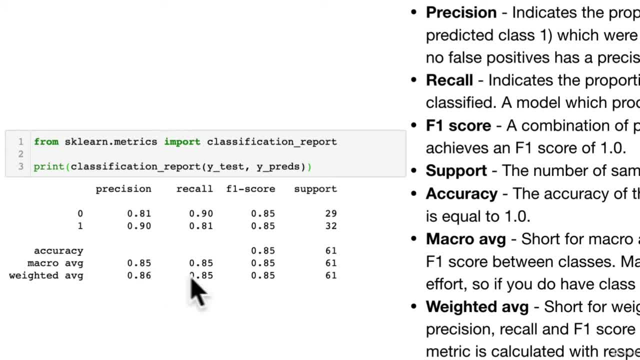 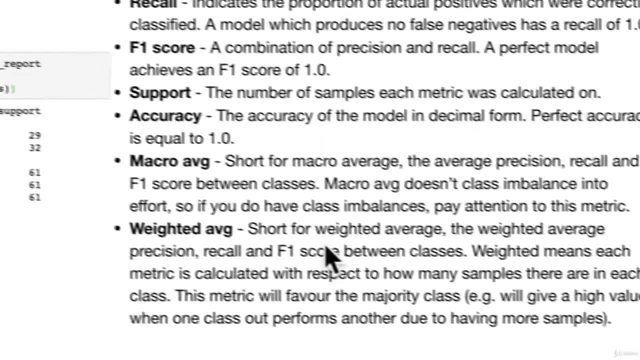 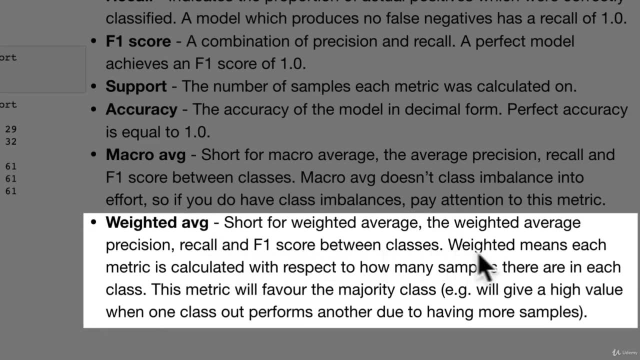 class imbalances. you really want to check out your macro average Now because our example, the classes are relatively balanced. that's why the macro average and the weighted average short for weighted average AVG. the weighted average is the precision, recall and F1 score between classes. Weighted means each metric is calculated with. 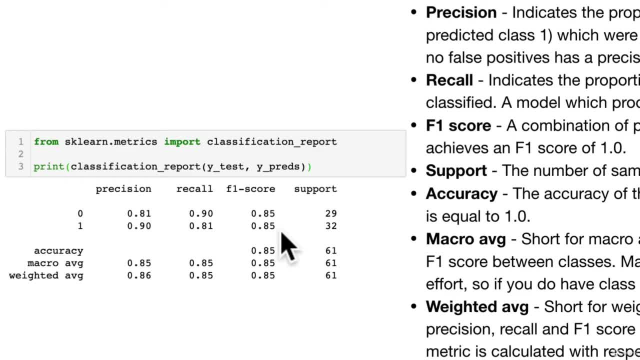 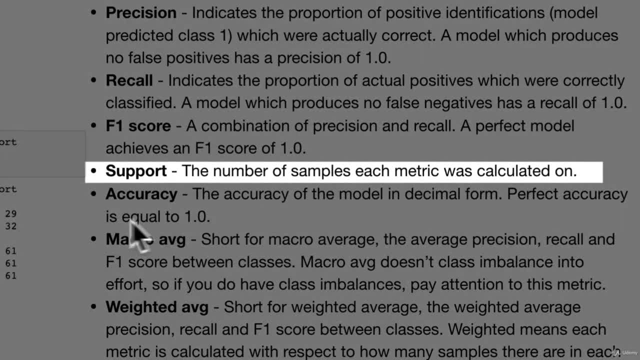 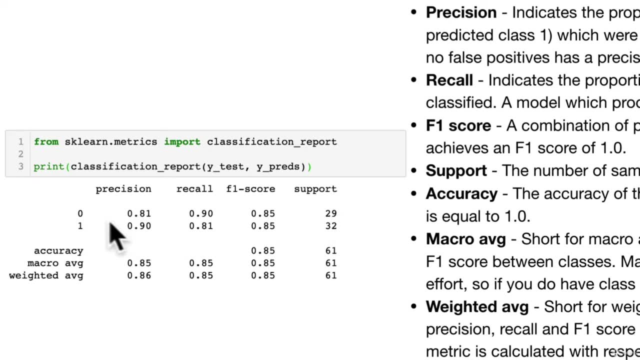 Okay, so we see our F1 score. That score is not 1.0, but it's still relatively high. Then if we go support The number of samples, each metric was calculated on. So we see here: So this means we look at this 29. So if we look at that, that's for zero. 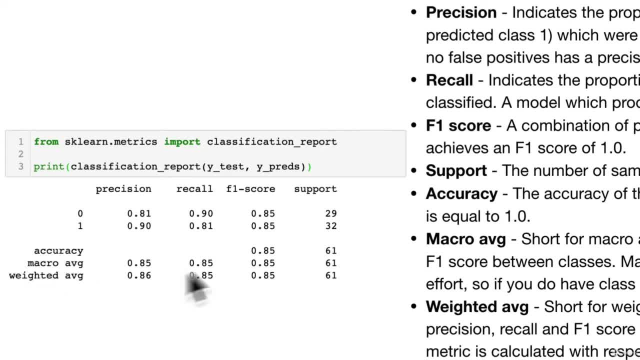 Down here it's 61. So that means that these metrics here were calculated on 61 different samples And these metrics along here were calculated on 29 samples which had the class 0, and that this one is 32 with the class label 1: aka has heart disease. and so if you total these, 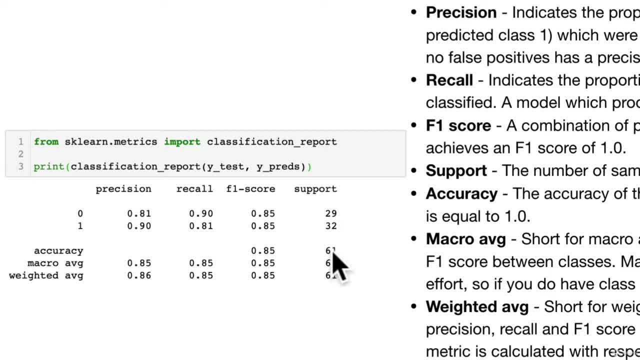 up 29 plus 32, you get 61.. Now accuracy. we've seen that before. this is just the accuracy of the model in decimal form. perfect accuracy is 1.0. aka our model is making predictions right 100% of the time if its accuracy is 1.0. Then we have a look at macro average. now what is that? it's short for. 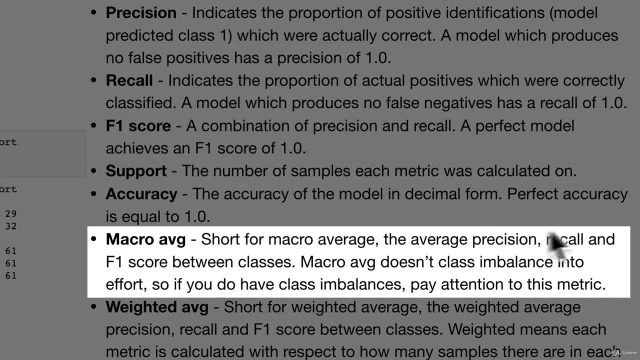 macro average, as you may have guessed. so it's the average precision, recall and f1 scores between classes. Now the key here is macro average doesn't take class imbalance into. this should be effect into or account, so pretend this is account. so if you do have class imbalances, pay attention to this. 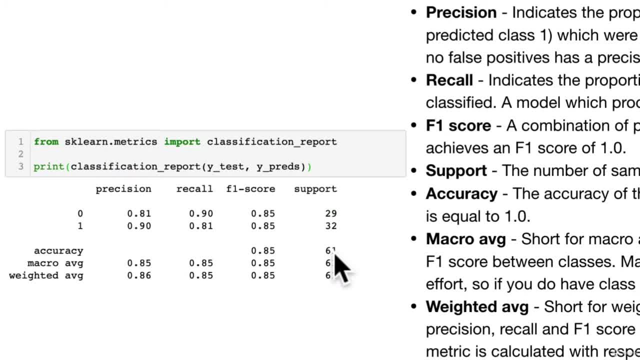 metric. Okay, so in our case, what does it class Imbalance? well, if you look at our example, we don't have class imbalances here. why is that? well, because we have relatively the same amount of samples with class 0 and class 1, meaning we've 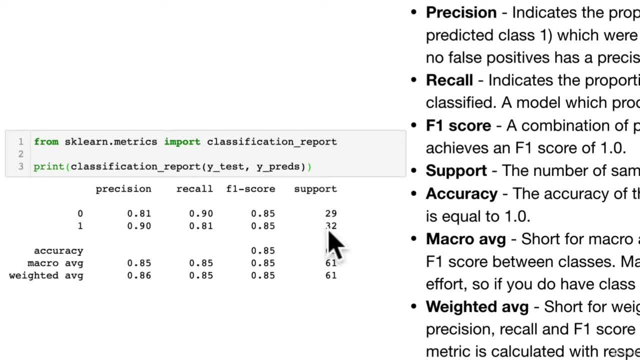 got about 50- 50 split here. it's not exactly 50- 50, but it's not like we have 60 examples of class 1 and 1 example of class 0, so we've got about 30 in each. so if you did have class imbalances, you really 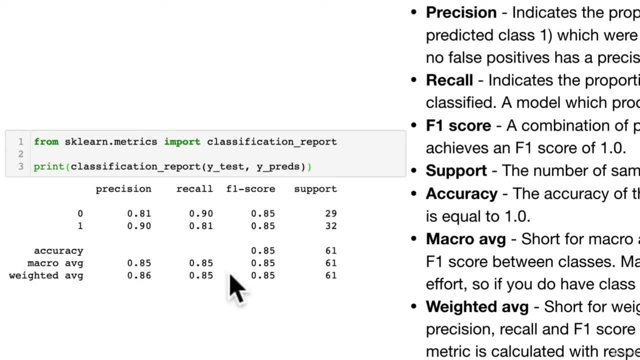 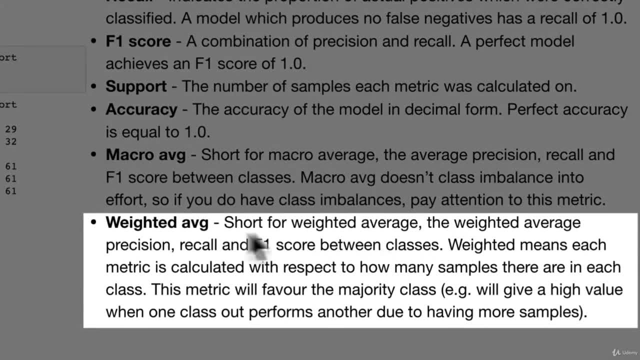 want to check out your macro average now, because our example- the classes- a relatively balanced. that's why the macro average and the weighted average short for weighted average AVG. the weighted average is the precision, recall and F1 score between classes. weighted means each metric is calculated with respect to how many samples are in each class, so this metric will favor the majority. 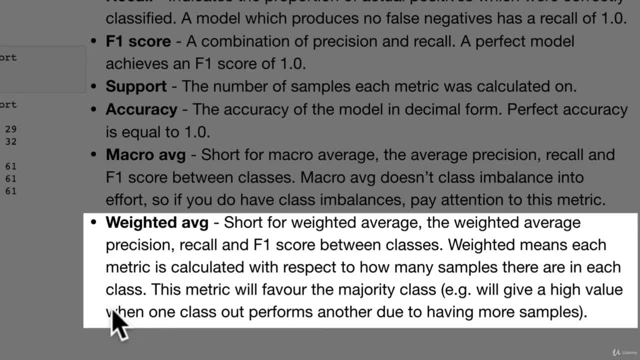 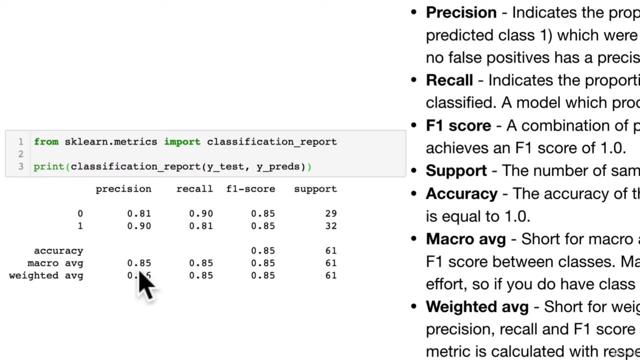 respect to how many samples are in each class, So this metric will favor the majority class. For example, we'll give a high value when one class outperforms another due to having more samples. So this is why that our values here are quite similar. 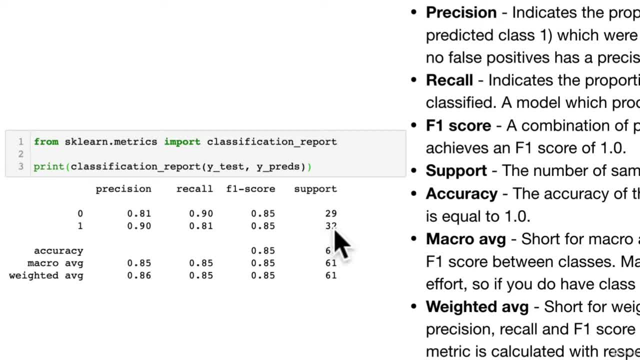 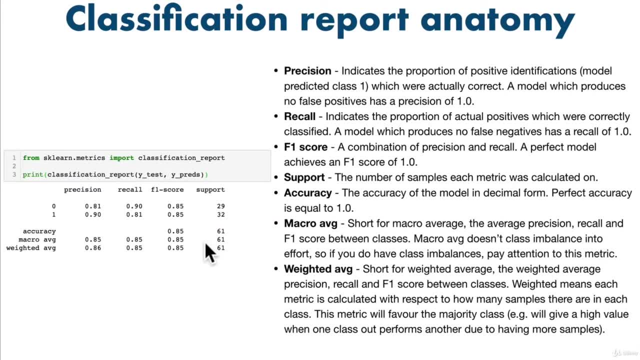 Because we have balanced classes. Now you might be thinking: is what kind of situation would it be that these values would be out of whack, right Like, where would this happen? And you might also be thinking: we've learned a whole bunch of different metrics here We come back to our 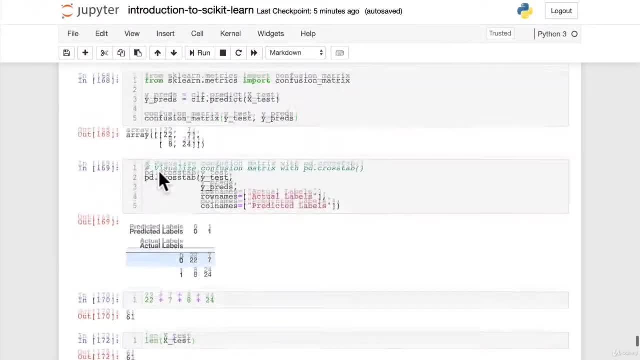 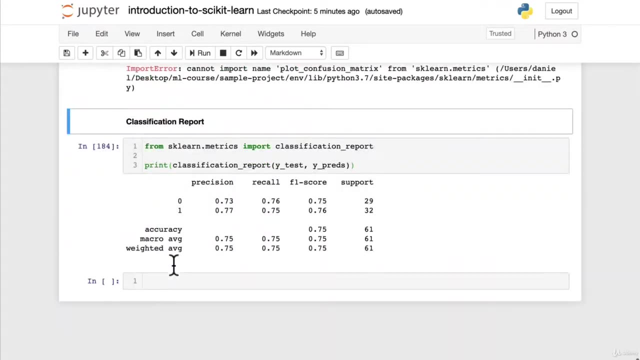 notebook. We've gone over classification reports, We've done confusion matrix, We've done accuracy, We've done area under rock curve. So when should I use each of these? So now we've kind of gone through them. It might be tempting to think: well, why don't I just 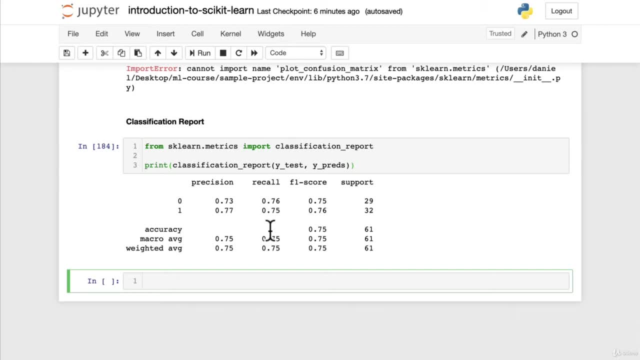 switch all these other ones that I really am having kind of trouble grasping and just use accuracy. Well, let's have an example, Let's see when other metrics come into play, and maybe you shouldn't just use accuracy, Because this is a trap that I got caught in right When I first started building. 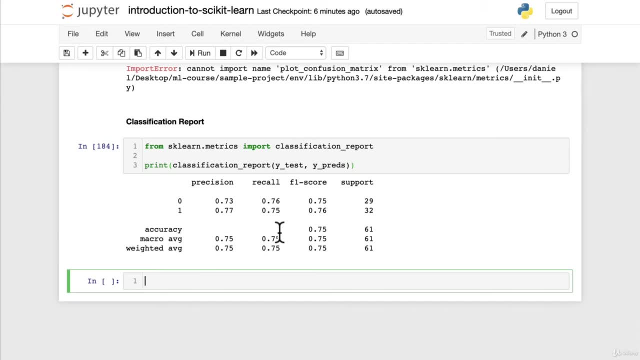 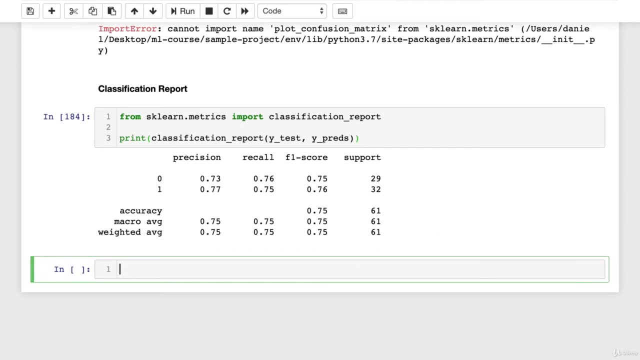 classification models, I was like, yes, my model is getting 90 plus percent accuracy. It must be a great model. Let's see a scenario So, for example, let's say there were 10,000 people and one of them had a disease and you're asked to build a model to predict. 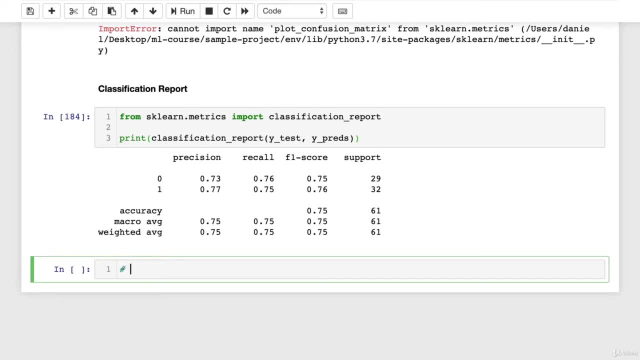 who has it All right. So let's actually do that, Let's code this up. So this is where precision and recall become valuable, And, in fact, all the metrics in our classification report become valuable here. So disease, true, So there was 10,000 people and one of them had a disease. So what we? 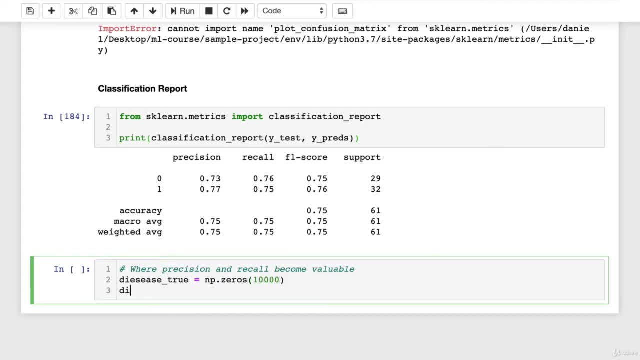 might do is create an umpire array of 10,000 people And then we might change one of these. I can spell disease, So disease zeroth index equals one, So there's only one positive case. Then if we come down here and say our model predicted or disease preds equals NP zeros. 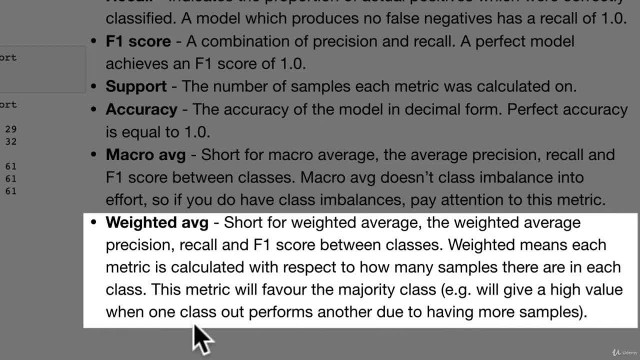 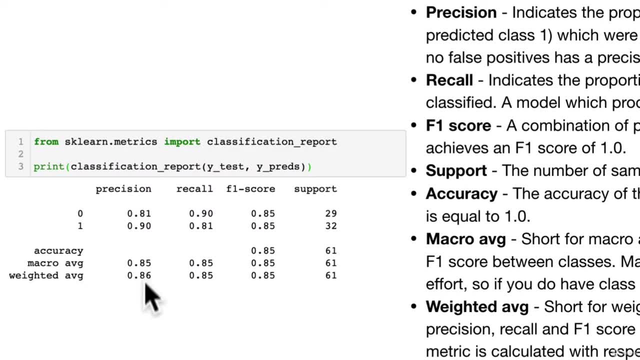 class, for example, we'll give a high value when one class outperforms another due to having more classes, more samples. so this is why that our values here are quite similar, because we have balanced classes. now you might be thinking is what kind of situation would it be that these values would be? 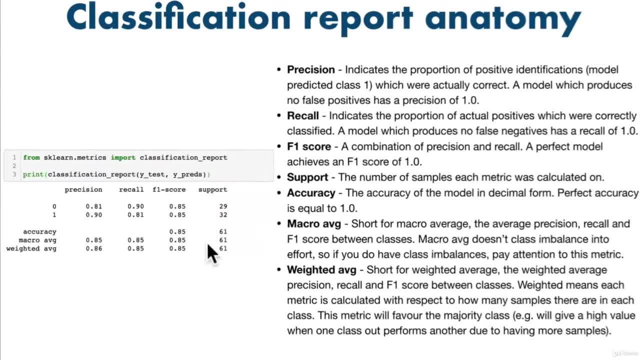 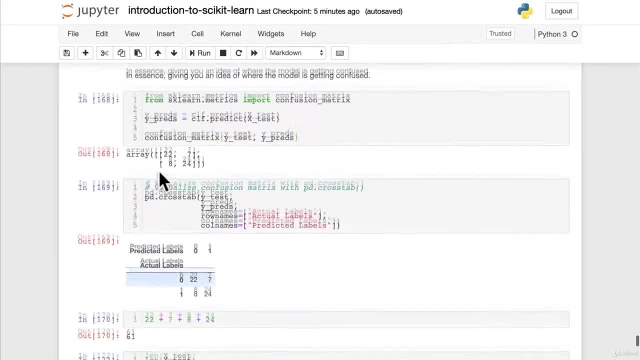 out of whack, right like where would this happen? and you might also be thinking: we've learned a whole bunch of different metrics. here we come back to our notebook. we've gone over classification reports, we've done confusion matrix, we've done accuracy, we've done area under rock curve. 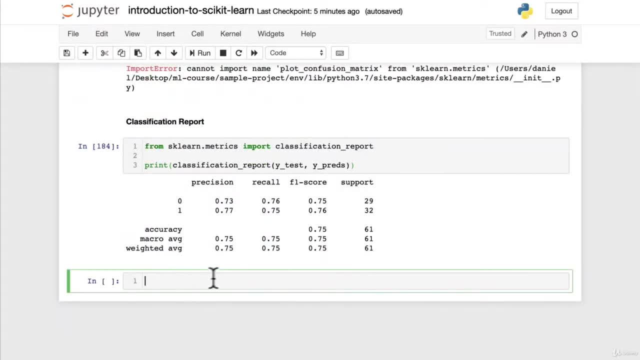 so when should i use each of these? so now we've kind of gone through them. you might be tempting to think: well, why don't i just ditch all these other ones that i really i'm having kind of trouble grasping and just use accuracy? well, let's have an example. let's see when other metrics come. 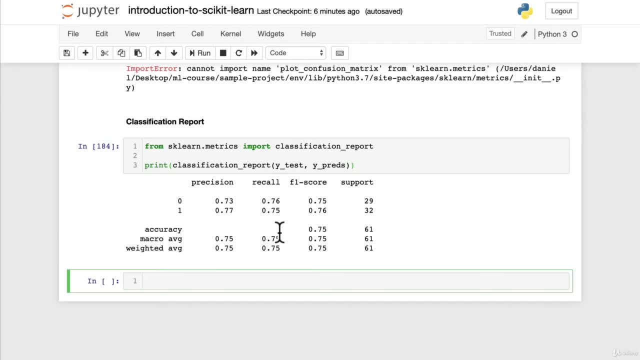 into play and maybe you shouldn't just use accuracy, because this is a trap that i got caught in right. when i first started building classification models, i was like, yes, my model is getting 90 plus percent accuracy. it must be a great model. let's see a scenario. so, for example, let's say there were 10 000 people and one of them had a. 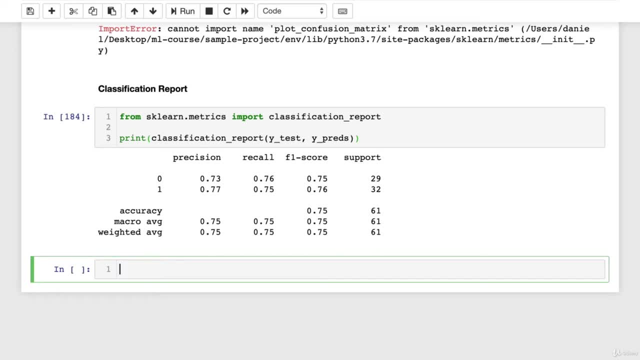 disease and you're asked to build a model to predict who has. it all right, so let's actually do that. let's code this up. so this is where precision and recall become valuable and, in fact, all the metrics in our classification report become valuable here. so disease true, so there. 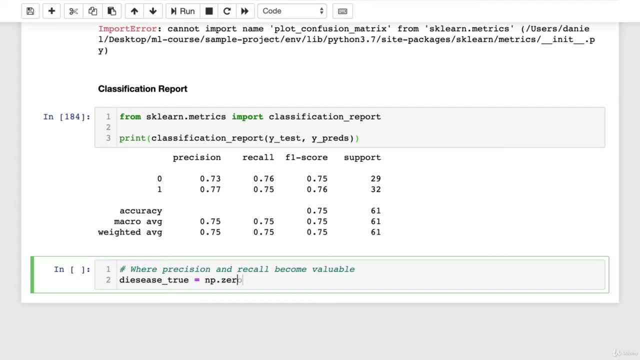 was 10 000 people and one of them had a disease. so what we might do is we might go ahead and create an umpire array of 10 000 people and then we might change one of these, if i can spell disease. so disease zeroth index equals one, so there's only one positive case. 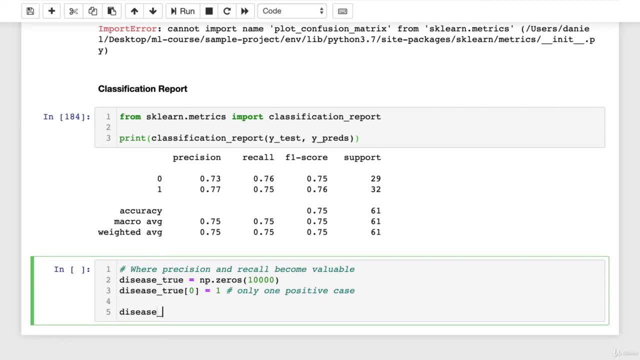 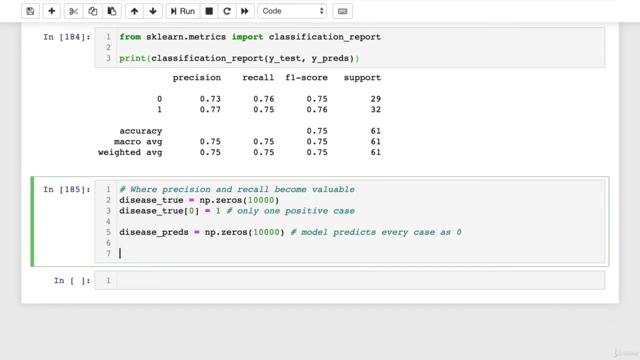 then if we come down here and say our model predicted or disease preds equals np zeros ten thousand. now, this means model predicts every case as zero, all right, and then what we're going to do is create a pd data frame so we can visualize this classification report. what if that's what our model did? right? 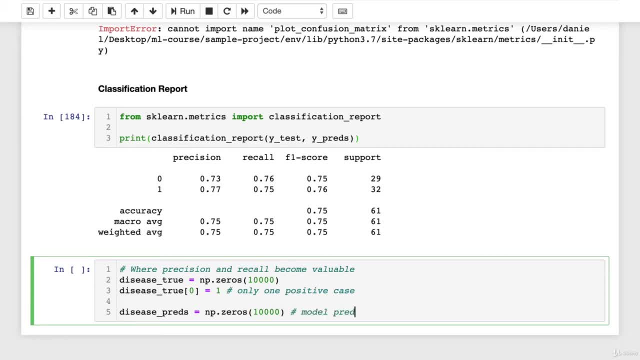 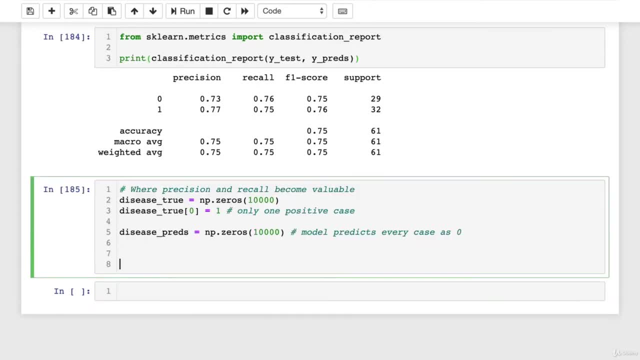 10,000.. Now this means model predicts every case as zero. All right, And then what we're going to do is create a PD data frame so we can visualize it. Classification report: What if that's what our model did? right? This is what's happening here. 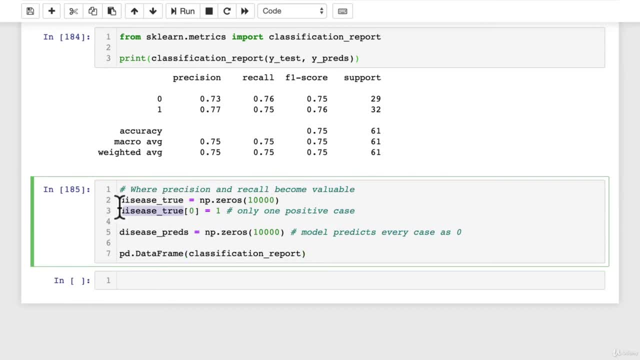 Disease. true, So there's only one positive case, one in 10,000.. And we build a model and our model predicts that every single case is zero, So it misses the one prediction. What would happen if we build a classification report? So we go disease. true, We go over here. Disease preds. 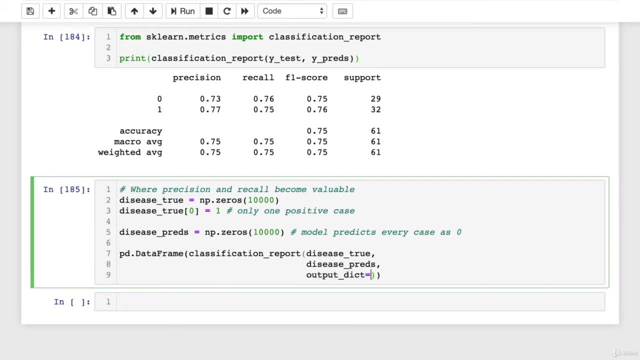 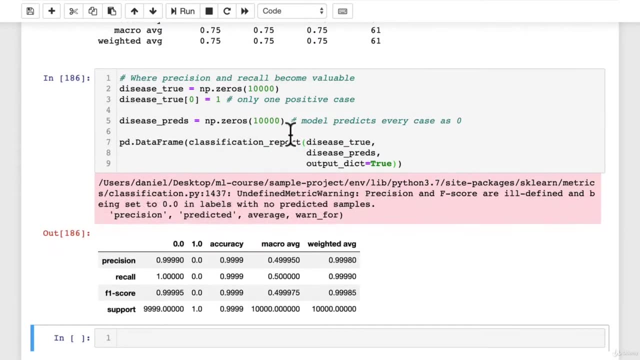 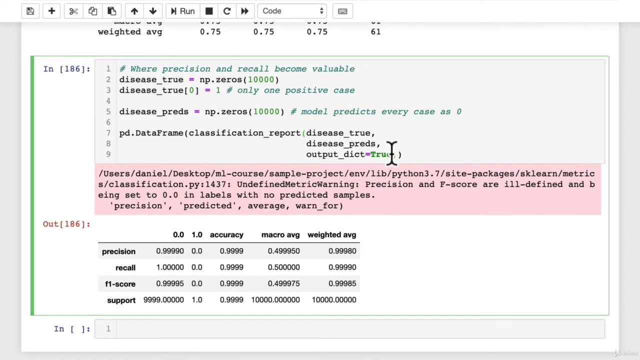 We want to pass this little parameter so it fits nicely into our data frame. So output dict equals true, All right. So what's happening here? If we look at this, this is just another format of this classification report up here. If we didn't do this, 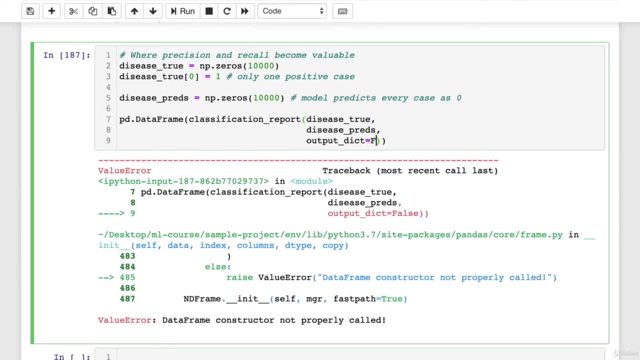 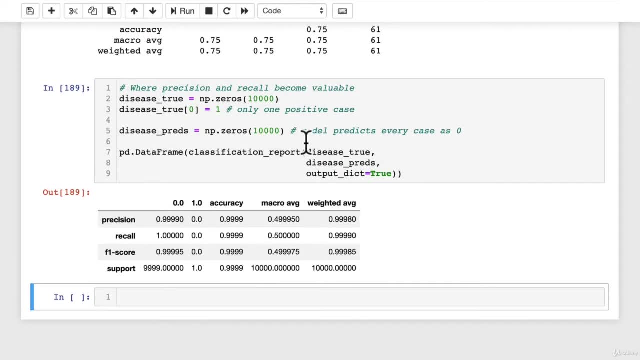 it would error out. So this is just to visualize what's going on, True? So this is a prime example right of where you want to use another metric other than accuracy, It's when you have a very large class imbalance. So in our case, we have a massive class imbalance. 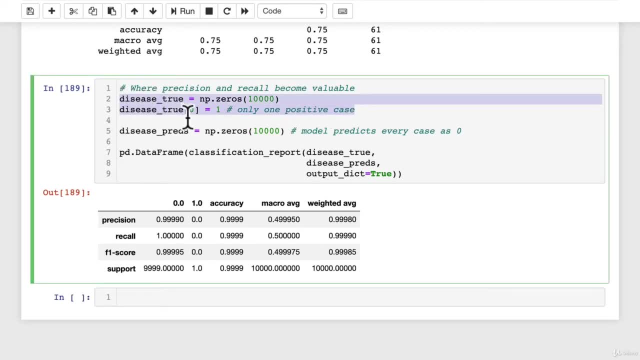 because in our original data set, disease equals true. there's only one example, So only one example of where the label would be one and everything else is zero. We've built a model that just predicts zero for every case, right, Because it's only one sample. So it's really. 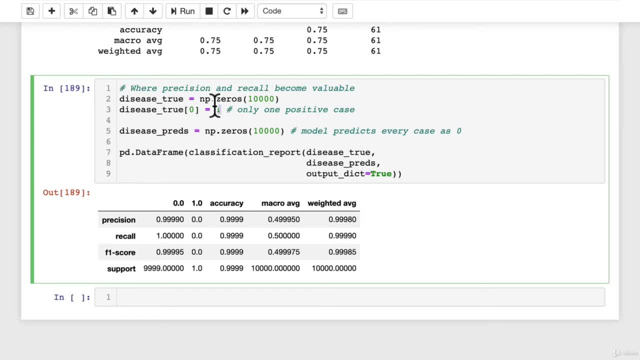 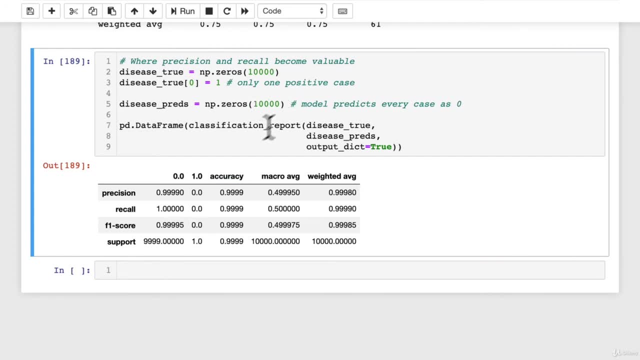 hard to learn that there's a pattern there for this one particular case, And so what happens is, if we were to measure just accuracy on our model, we're going to have a very large class imbalance. We're going to have a model that is predicted zero for everything. It comes out with an accuracy. 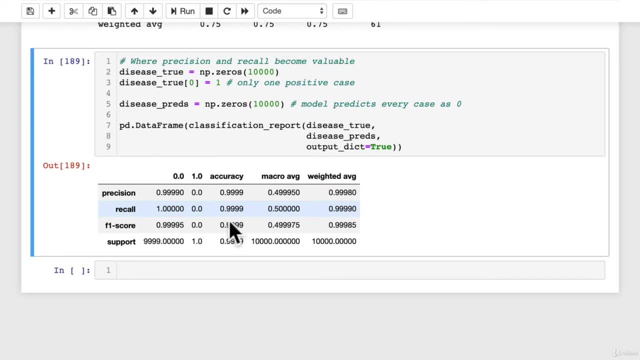 of 0.99, or in other words, 99%. And so ask yourself: although the model achieves 99.99% accuracy, is the model still useful, right? That's where we look at these other metrics, such as the macro average. That's where we can see, okay, our model's falling down here. 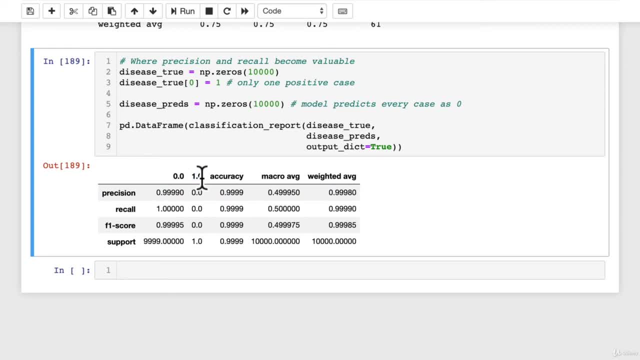 on the precision, It's actually getting zero precision for class one, which makes sense for class one, And here it's getting basically 100% on class zero because it has only predicted class zero. So this is a kind of use case scenario of where you want to make sure that you're using 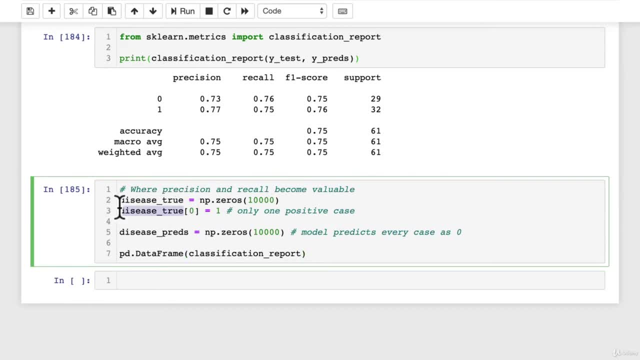 this is what's happening here: disease, true. so there's only one positive case, one in 10 000- and we build a model and our model predicts that every single case is zero, so it misses the one prediction. what would happen if we build a classification report? so we go? disease true. 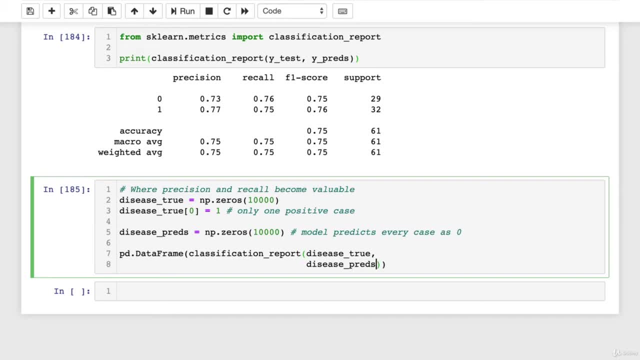 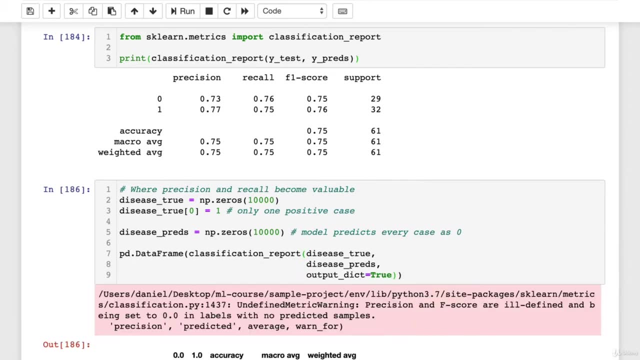 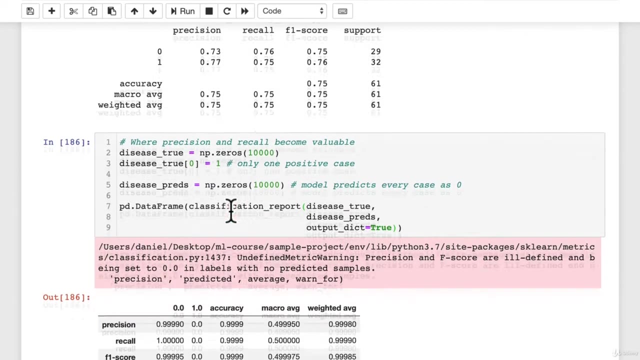 we go over here: disease preds. i want to pass this little parameter so it fits nicely into our data frame. so output dict equals true, all right. so what's happening here? if we look at this, this is just another format of this classification report up here. if we didn't do, 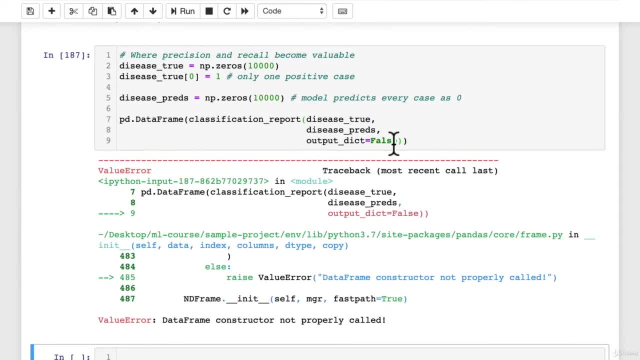 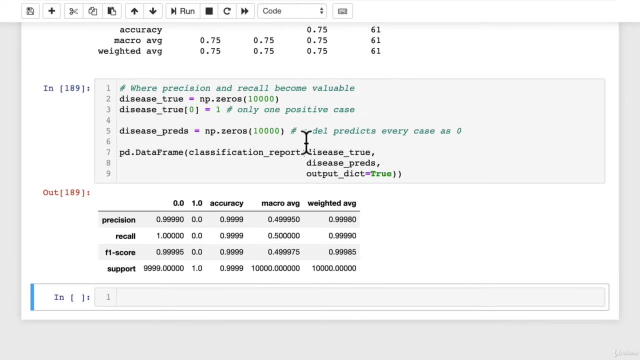 this, it would error out. so this is just to visualize what's going on, true? so this is a prime example right of where you want to use another metric other than accuracy is when you have a very large class imbalance. so in our case, we have a massive class imbalance because 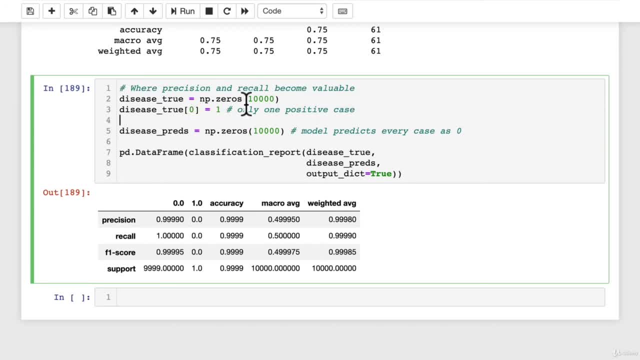 in our original data set, disease equals true. there's only one example, so only one example of where the label would be one and everything else is zero. we've built a model that just predicts zero for every case. right, because it just it's only one sample, so it's really hard to learn. 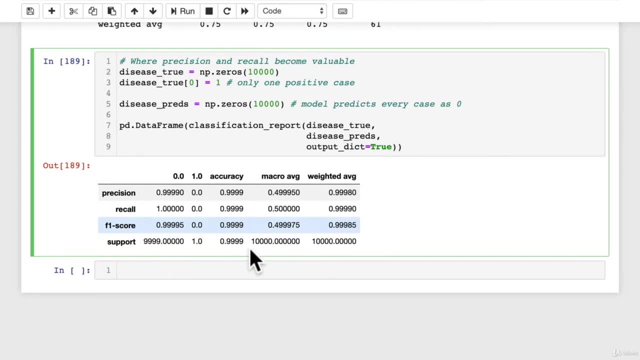 that there's a pattern there for this one particular case. and so what happens is, if we were to measure just accuracy on our model, that is predicted zero for everything, it comes out with an accuracy of 0.99, or in other words, 99 percent. and so ask yourself: although the model 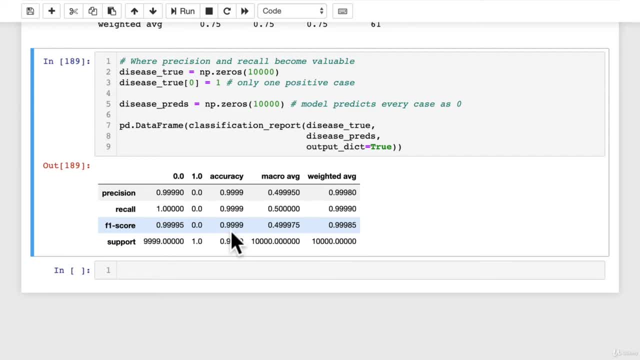 achieves 99.99 accuracy. is the model still useful? right, that's where we look at these other metrics, such as the macro average. that's where we can see: okay, our model is still useful. model's falling down here. on the precision, It's actually getting zero precision for class one. 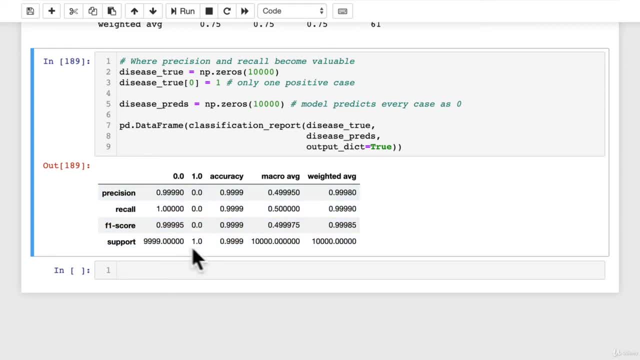 which makes sense, because it didn't even predict class one, And here it's getting basically 100% on class zero because it has only predicted class zero. So this is a kind of use case scenario of where you wanna make sure that you're using a wide spectrum of evaluation metrics.